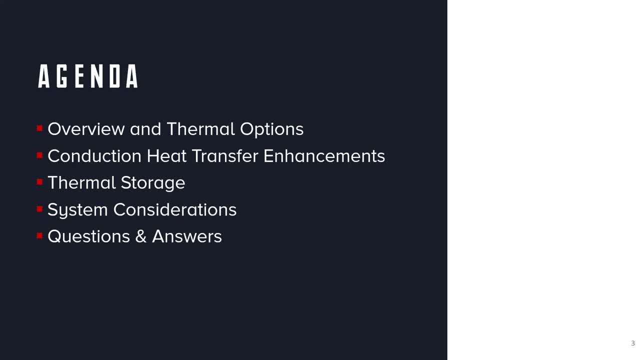 heat transfer enhancements, We'll talk a little bit about thermal storage and then we'll end just some high level on system level considerations and then we'll be happy to take your questions and hopefully go through some Q&A at the end. So again, please feel free to reach. 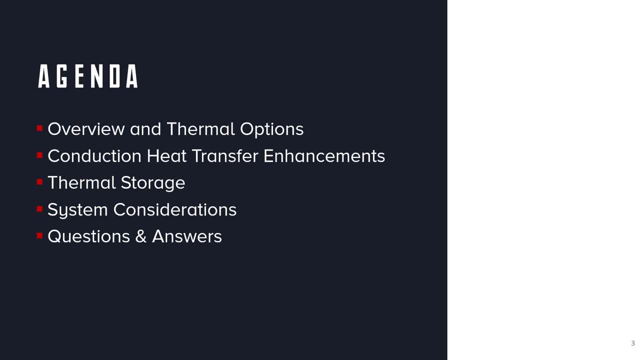 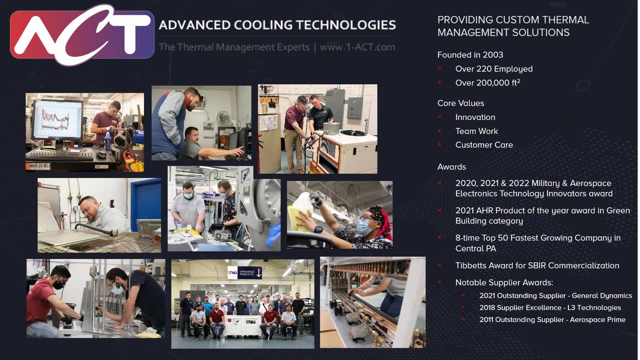 out and type in your questions or save them to the end, and we'll do some live Q&A. So for those new to advanced cooling technologies or haven't joined a webinar before, just a brief overview. I won't dive into too much detail, but we were founded in 2003,. 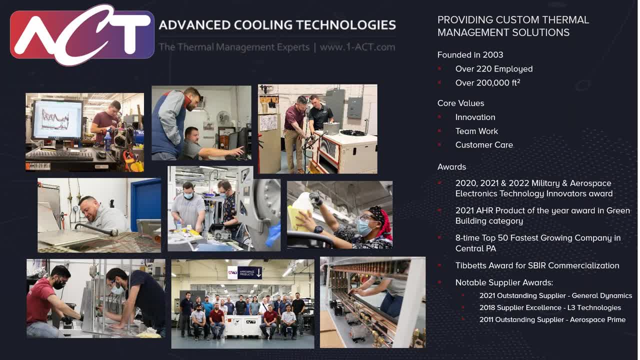 currently have over 220 employees and over 200,000 square feet. Our core values are innovation, teamwork and customer care. And just to highlight on some of the awards, the past three years we've won Military and Aerospace Electronics Innovation Award. 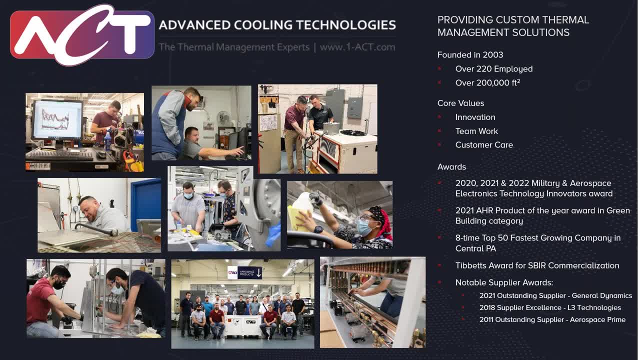 And a lot of the technologies we'll talk about today are actually recipients of that award. So, yeah, please feel free to reach out if you have any questions on anything not covered today. but we'll kind of focus in on some of those electronic schooling areas for aircraft. 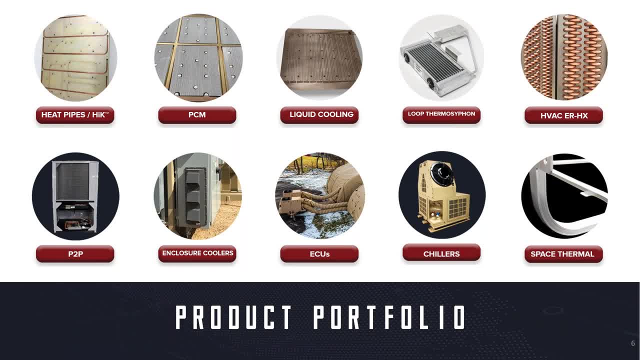 applications today And again we'll focus in on a couple of key technologies here, a lot on the component level- cooling with heat pipes, high K or high thermal conductivity cards, phase change material for thermal storage, and we'll just kind of briefly touch on system level considerations. But this slide is just to show kind of the larger. 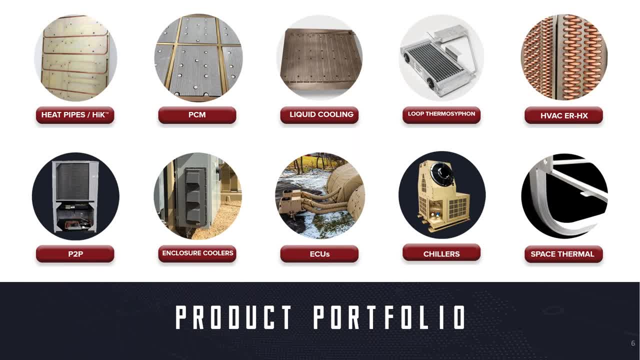 depiction of all the thermal options for various systems, aircraft and ground-based systems. So if you have any questions on things not covered today, again please feel free to reach out. We have a lot of good resources for any of these types of technologies. 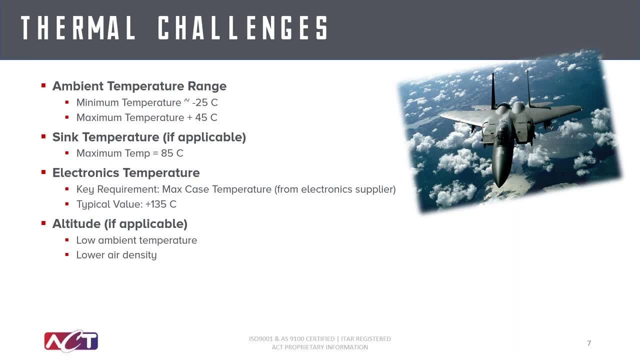 So let's jump into some of the thermal challenges associated with avionics cooling. The first one is the ambient temperature range, Typical for military environments and especially for aircrafts. you have a fairly wide temperature range that you need to design to. It can go all the way down to minus 25 and below. 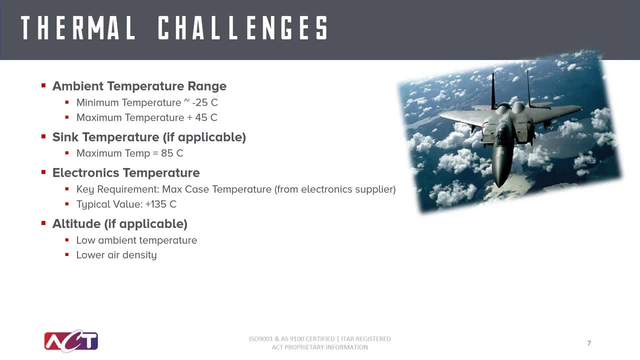 and it can exceed plus 45 degrees C. So a fairly wide temperature range and some pretty extremes going on for the ambient sink temperature design In terms of sink temperature. when we talk about sink temperature, it's not just the ambient air temperature. 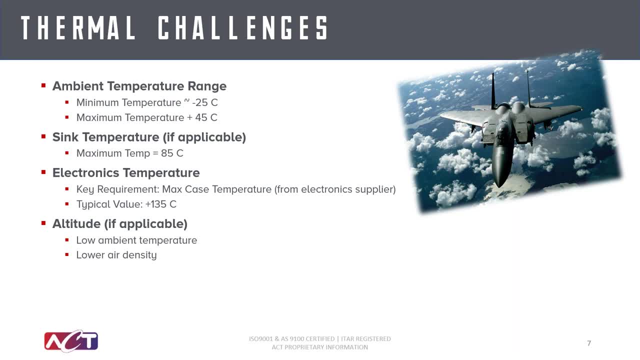 it's usually the design considerations. So for example, we have a lot of case resistance, But in most cases that's fairly well known from the electronics manufacturer. So we'll design to the max case temperature And again it's making sure that the thermal 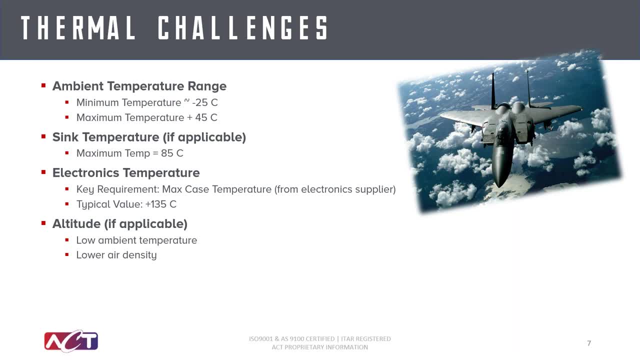 resistance network from the case to that sink does not exceed the thermal budget. So in this case we're saying a typical value is 135 degrees C for the case temperature. So that gives you a 50 degree budget if your sink temperature is 85 degrees C. And then some other considerations. 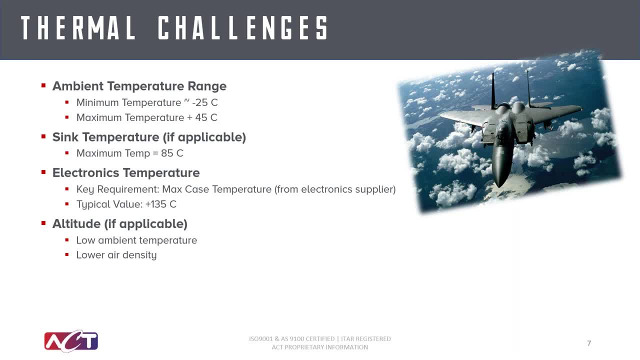 unique to aircraft is altitude, So in those cases where you have high altitude considerations, you might run into even more low temperature extremes. So you might have to design some residual power to make sure your electronics don't get too cold And you also have low air. 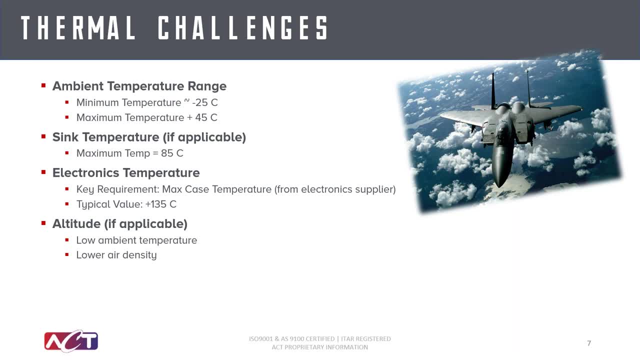 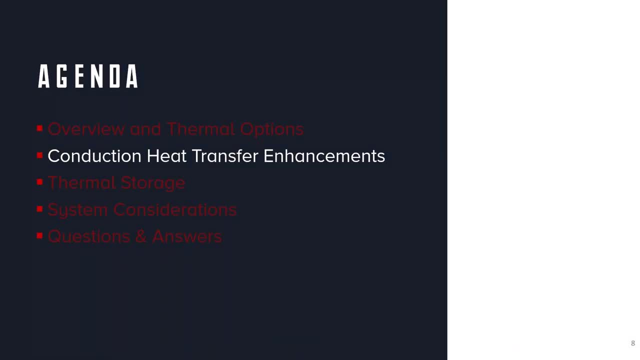 density. So you've probably got to design past just convective heat transfer and look at the radiation side as well if you have extreme low air density ranges. So with that, that's kind of just an overview Of the challenges. Now we'll talk about enhancing some of your heat transfer. So 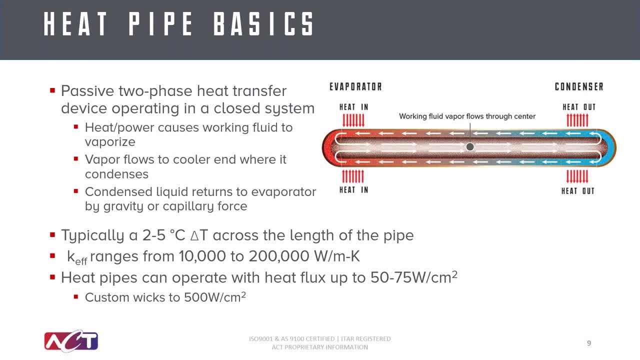 conduction. cooled systems are one of the most common for avionics. It's the most easy to design to If you can get away- if your power is low enough that you can get away with just metal conduction, that's obviously the easiest and most economical. But when that's not possible, 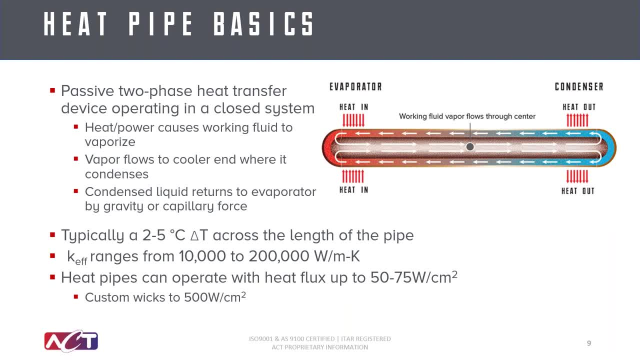 you look to enhance the conduction paths And there's a couple different options: unique materials, unique metals, Things like silver or diamond spreaders have been used, But one of the more economical ways is to use heat pipe technology. So if you're not familiar with heat pipes, we have a lot of resources. We'll just kind of dive into the high level overview of how these work today. 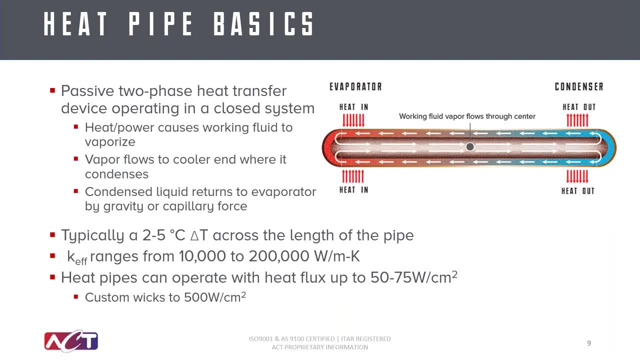 But if you're interested in more of either the theory or the practical side, we have a lot of resources online, including reliability guides, including a lot of the theoretical papers and things like that, But just to give kind of a brief overview. So just a brief overview of how they work. 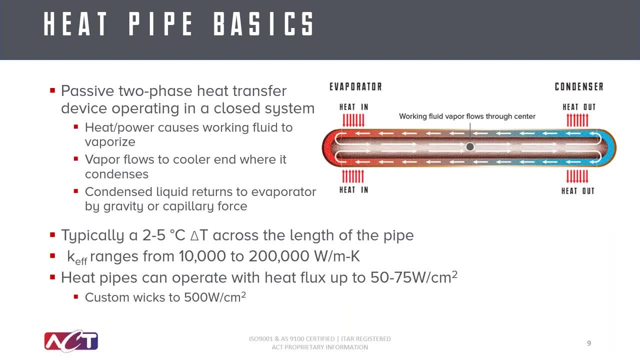 You couple your heat pipe to your source electronics and you couple one side to your sink And with that you input power with your electronics. it will vaporize the fluid, the working fluid inside the heat pipe. That will create a pressure gradient which will push the fluid to where it's cold in your system. 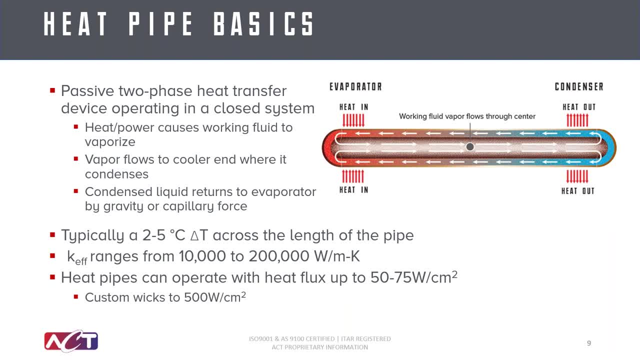 When you couple that side to the heat sink, the fluid will give up its latent heat, return back to a liquid, And then it's absorbed into a wick structure which lines that fluid, the ID of the pipe, And that wick structure creates a passive capillary force. 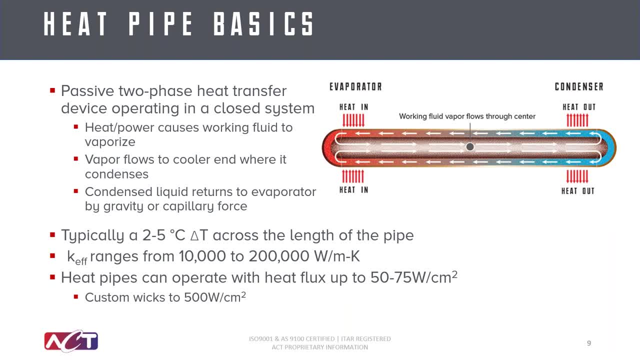 which then pumps the fluid back to the hotter source of the evaporator area. So completely passive, no moving parts. It's all created with the wick structure and the pressure fields And overall you get highly efficient heat transfer. So you move from point A to point B. 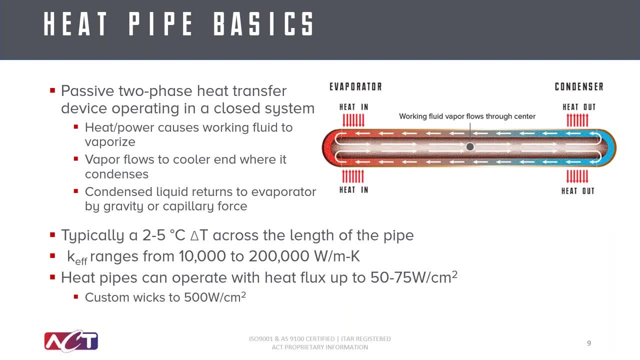 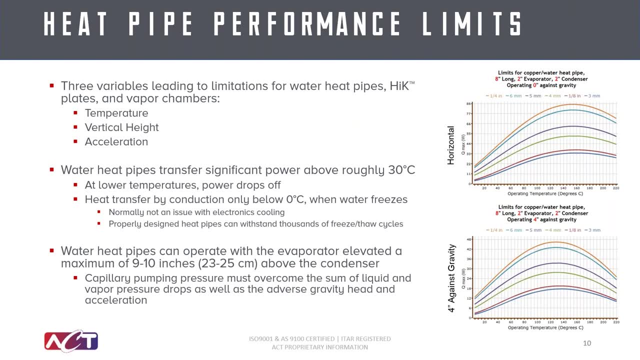 with less than a five degree temperature difference, So that can really short circuit your heat transfer path from your source to your sink when implemented properly. And just to talk on some of the limitations, one of the big design criteria for heat pipe is making sure that the heat pipe, or heat pipes- 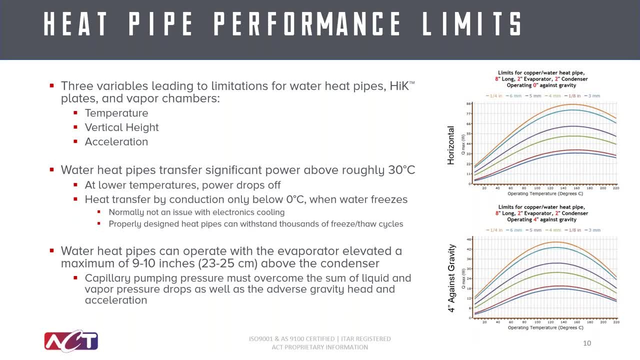 in your system have enough capacity to move the entire heat load. So some of the considerations there is the temperature range. We'll talk mainly about water heat pipes today because the temperature range we talked about at the max case temperature or sink temperature within that heat pipe. 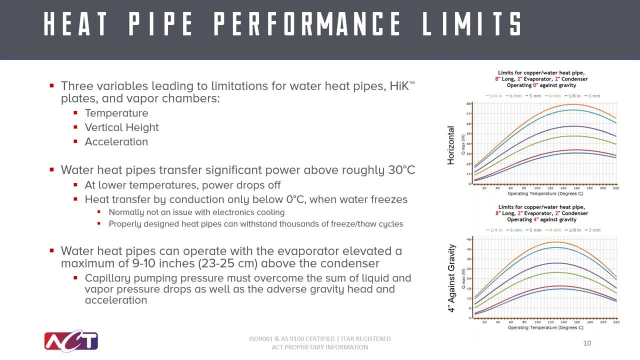 within that 85 to 135 degrees C range, water is the optimal fluid choice for those type of systems. So we'll talk mainly about water today, but there are other working fluid options if you have different extremes in your temperature ranges. But temperature is one of the main criteria. 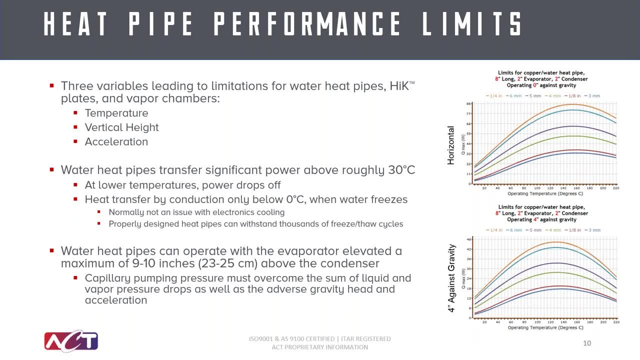 Vertical height. that is the orientation of the heat pipe with respect to gravity. So if you have to pump using the wick structure to create that capillary pumping action, if that is against gravity, then it's a little, a little harder to pump against gravity. 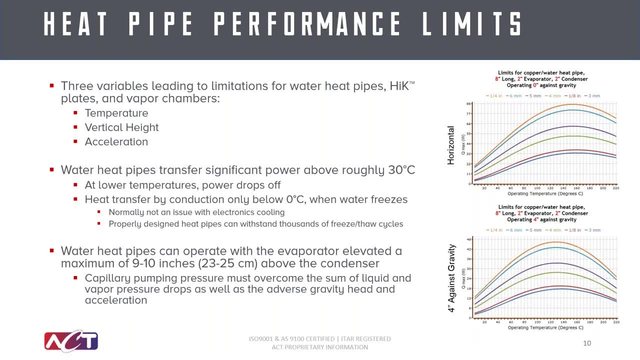 with the different pressure drops in the system. So that's a design criteria we need to take into account. And then, specific to aircraft applications, acceleration. If you have different acceleration fields that you need to design to, again, we need to take those into account. 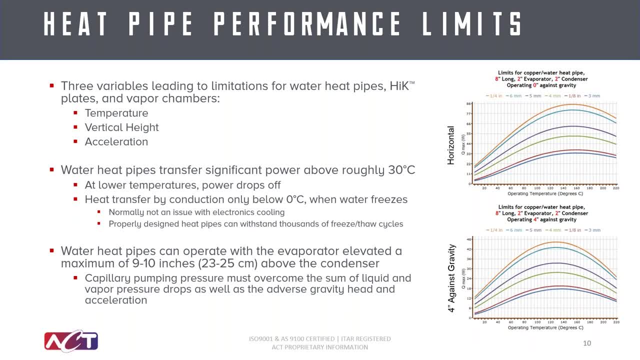 and make sure that we design and model to those situations. So looking at the curves we're showing here, you can see that water heat pipes can move a significant amount of power above kind of the 25 to 30 degrees C range. So if you get too low in temperatures, 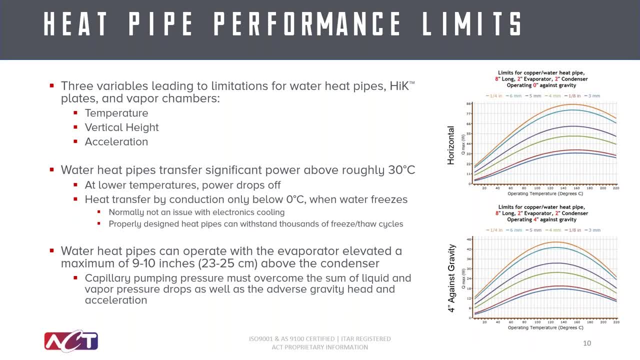 water will, as you get closer and closer to zero water, will freeze. It'll survive freezing, but it won't operate during freezing, So you'll be able to survive and keep your electronics from overheating during the frozen conditions, based on the secondary conduction paths. 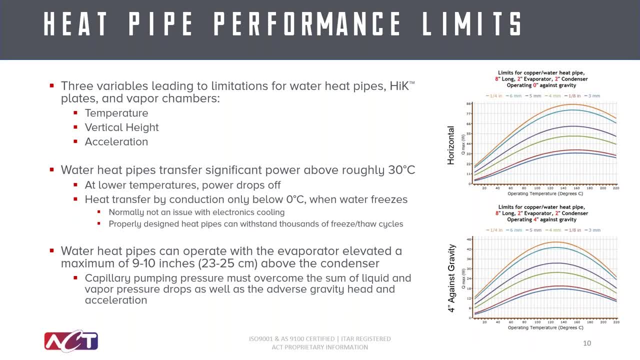 And then, as your heat pipes will heat up, it'll start transferring power as you get closer to the key temperature ranges, closer to your extremes, And it just kind of talking about this according to the vertical height or the orientation with respect to gravity. 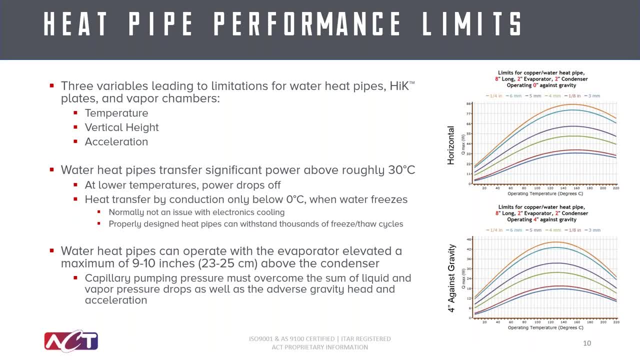 the two plots we're showing on the right. the first one is horizontal operation And then the second one is with a short distance against gravity. So you can see how it kind of changes the capacity of the heat pipes in those systems. But in either case we can design against gravity. 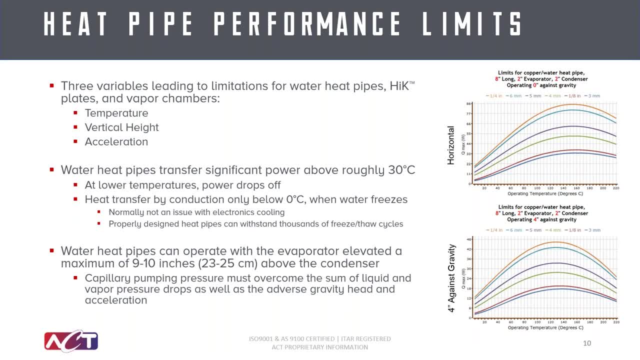 horizontal or gravity assisted. It's just a matter of properly sizing your heat pipes- both the diameter and the number of heat pipes in your system- to make sure you have enough capacity to move the entire heat load. And I'll start talking about some of the practical applications. 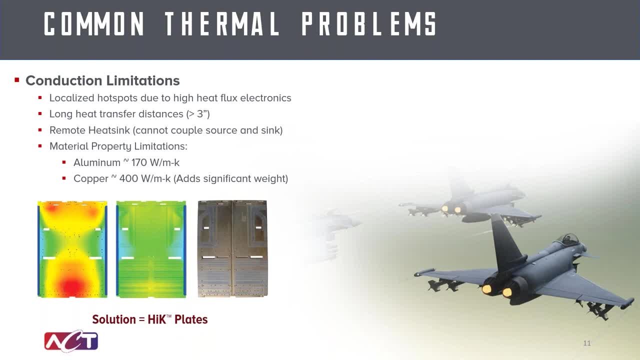 So one of the big challenges is conduction limitations. So the most common for avionics is aluminum that has roughly 167, 170 watts per meter K thermal conductivity. If you wanted to go to a higher thermal conductivity, metal copper is usually next selection. 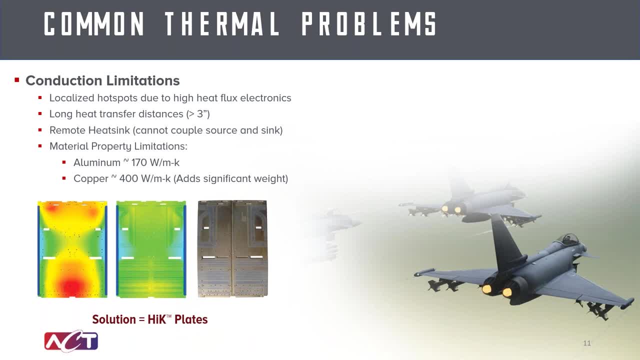 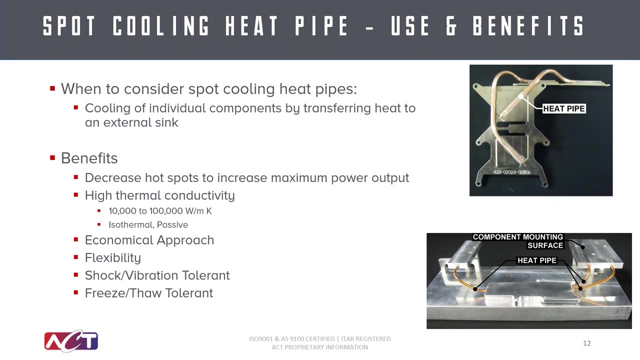 However, for avionics, where mass is a big concern, copper does add a significant amount of weight. So a lot of times our designers are trying to get the lightest weight, highest performing thermal solution. So, talking about spot cooling, the couple of different strategies in using heat pipes- 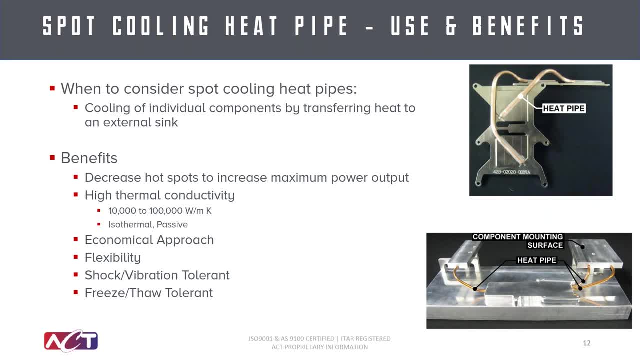 one is spot cooling, basically moving heat from point A to point B, point A being your electronics and point B being your sink- And in this case, if you're moving it short distances or you know you're moving it to a higher temperature. 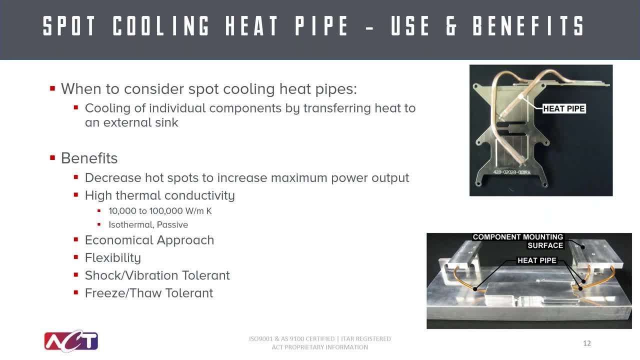 you're moving it to a higher temperature. You know you're moving it to a higher temperature And if you're moving it to a lower temperature, you're moving it to a lower temperature. unhealthy twostarted system will do that. 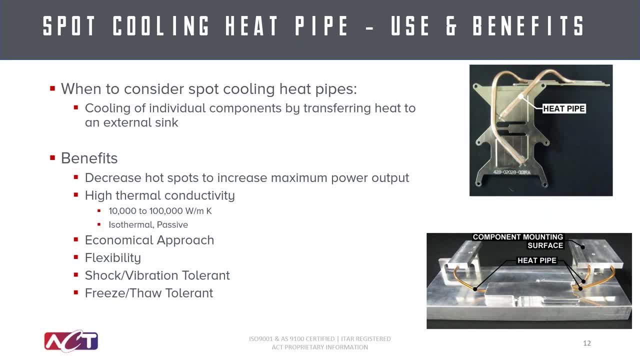 The third thing is constant heat and you'll notice that if you actually useful say for, say for combustion, then you'll- I use the Elizalde one so you'll notice that if you do a strengthen in Kotor Producer band. 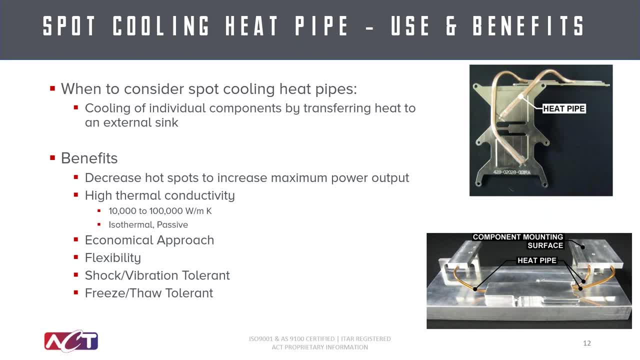 you can actually do that sort of interesting. Each Love concept thatquier would baked transfer tubes into you kind of a base here, three charging stations, sources and to a liquid cold rail which you can see kind of in the horizontal section above the the electronics there. but a pretty straightforward application. it was about 25 watts per square there. 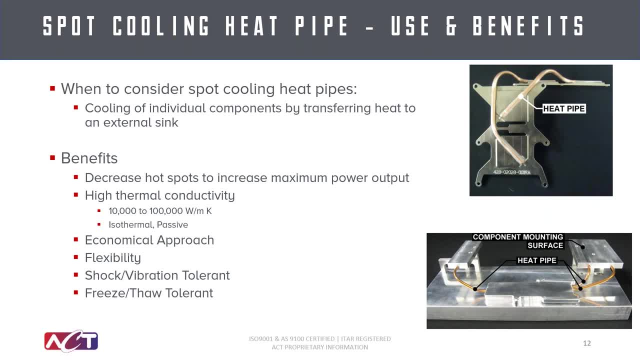 and we're just moving it from point a to point b and again you really cut down that thermal resistance because you're getting all the heat from source to sink with about a five degree temperature difference and then accounting for some of the metal conduction through the base. 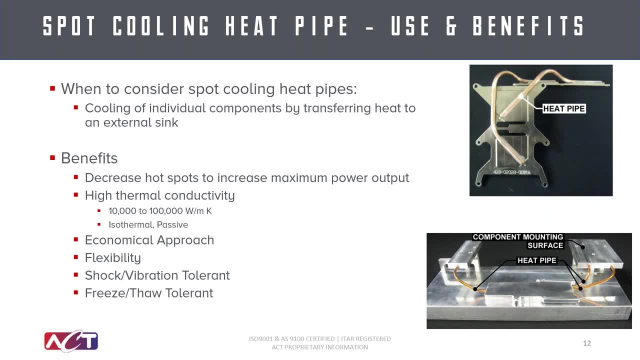 place. but the benefits here is the thermal efficiency that we talked about really drives down those case temperatures by short-circuiting the thermal path. but it's also a very economical approach. heat pipes are inherently low cost. it's copper tubing with some wick structure that we 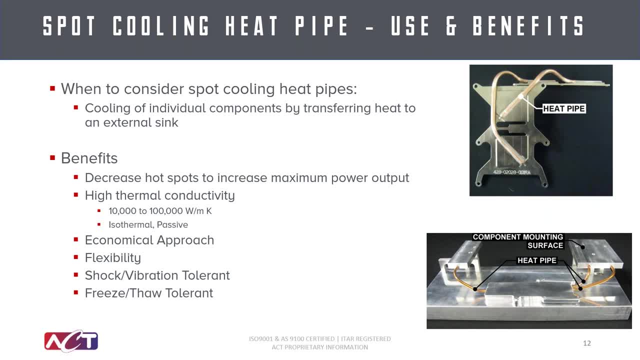 implement seal and there's not a lot of challenges in integrating these parts. having a good thermal joint is extremely important, but it's not a huge cost driver. it's just a kind of manufacturing know-how to make sure you have a really solid joint there. and again, they can be very flexible, easy to retrofit into designs and they are applicable. 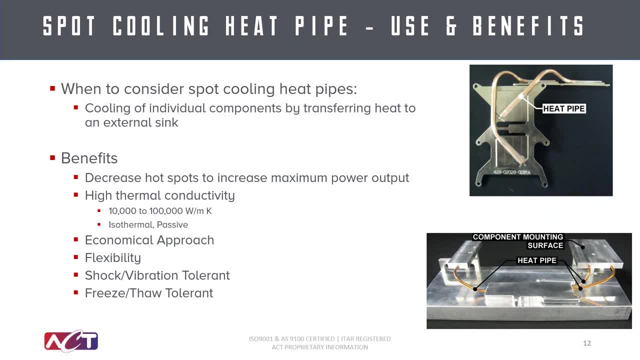 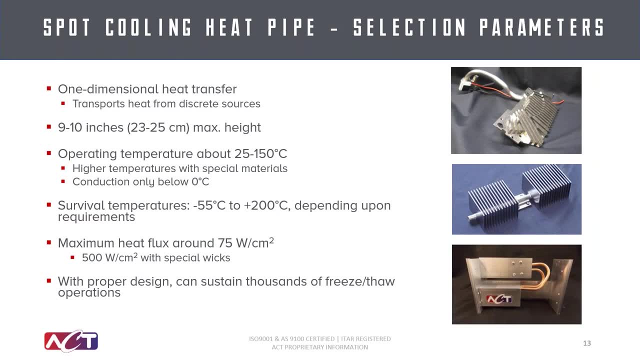 to all avionics mil standards, so they're shock tile and vibration tolerance and they can survive free stall and low temperature extremes as well. now looking at some of the the other spot, cooling advantages or limitations um the. the transport distance is one thing we we touched on a little bit, but 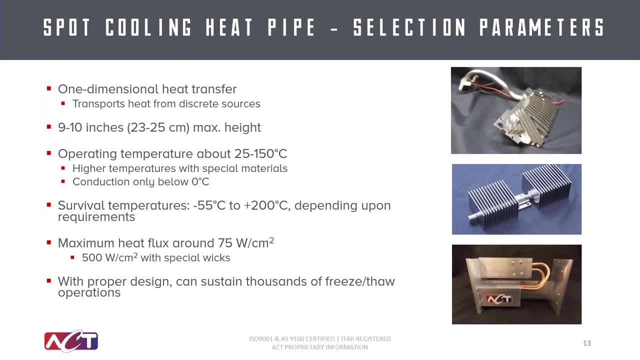 trying to limit the, the max height against gravity, to about 10 inches, is is one of the keys. so that's where you start kind of limiting your, your power capacity pretty significantly. again, it's a design consideration that we can take into account and see exactly how far we can transfer the, the heats. 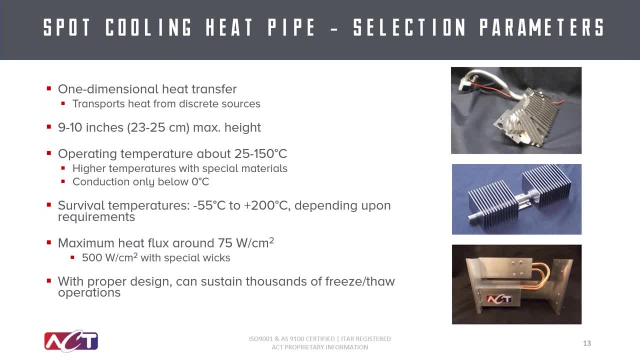 running some, some calculations, but general rule of thumb, nine to ten inches is a good maximum transport distance for this type of system. so the operating temperature range: i'm going to go into that in a moment. but the operating temperature range we talked about the low end on the. on the high end 150 is kind of a. 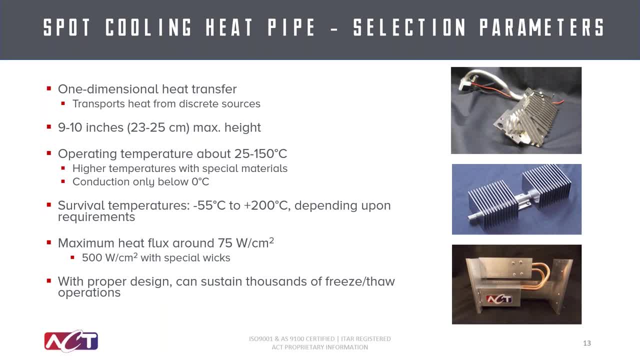 typical um design point that we'll- we'll go into that- exceeds by with some margin the max case temperatures that we're typically designed to from a survival standpoint. they can go up to about 200c. that's where the saturation pressure of the water becomes too extreme that it'll vent the heat pipe. 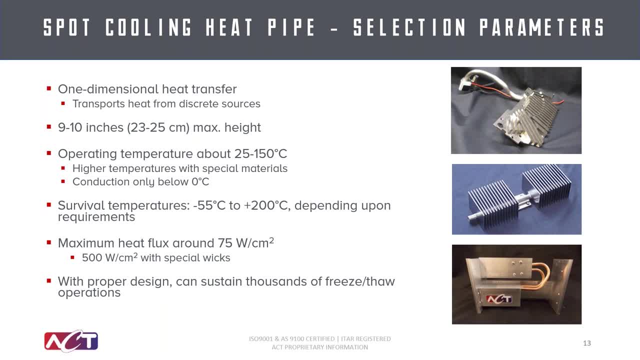 but again, if you're operating at that temperature or something probably has gone wrong in your system, you're running into some overheating electronics. already, from a max heat flux standpoint we typically say 50 to 75 watts per centimeter squared, which exceeds most avionics on electronics. 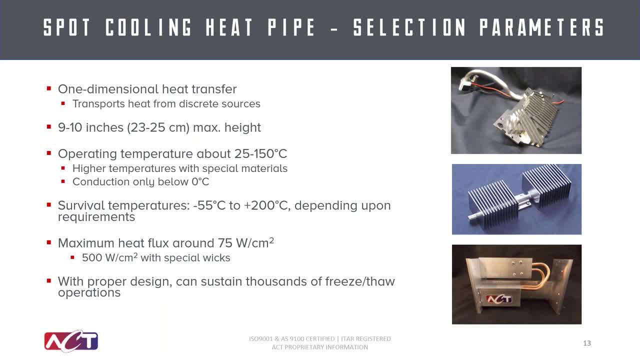 so usually we don't run into heat flux limitations in avionics applications, but if you do have really unique or high heat flux, we have done special wicks and cannot braid over 500 watts per centimeter square. and just touching on one of the designs, we'll talk about the top right one. this was: 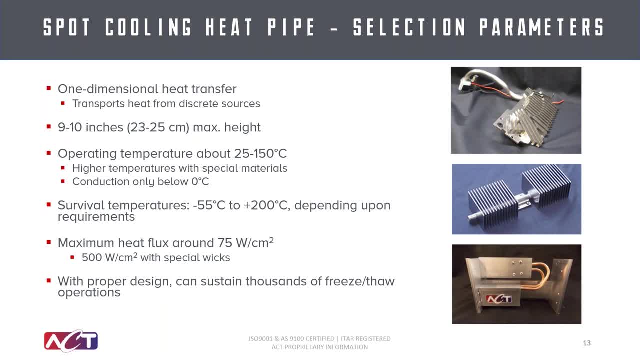 a avionics pod that was attached to beneath an aircraft, and this one had a unique sensor that needed to hold temperature for sustained operation. so it used a thermoelectric- the black square you can see there to the top left. that held temperature at about 25 degrees c and if you've used 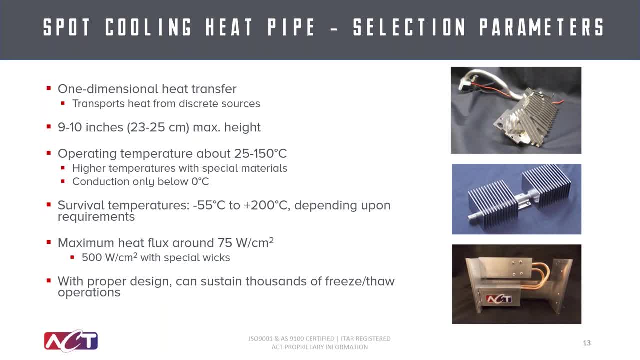 thermoelectrics before you know they're. they're somewhat inefficient, so holding temperature there with with the extreme environment around, you're dumping a lot of heat off the back side of the thermoelectric and that's where we took the heat pipe. they didn't have a large enough volume for. 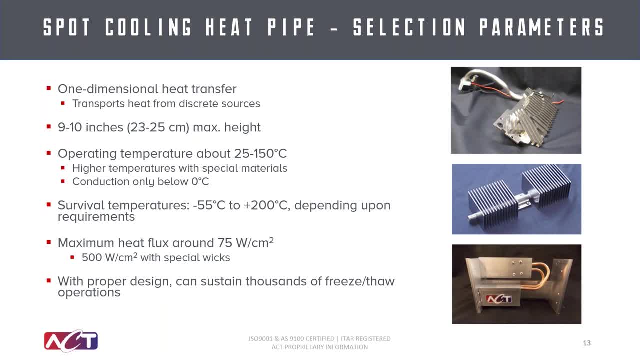 a heat sink right behind that. so the heat pipes just taking it to a remote heat sink where they did have some volume for air cooled. so a pretty straightforward application. you can see that the bends in the heat pipe pretty unique, just avoiding other components in the system. but again the 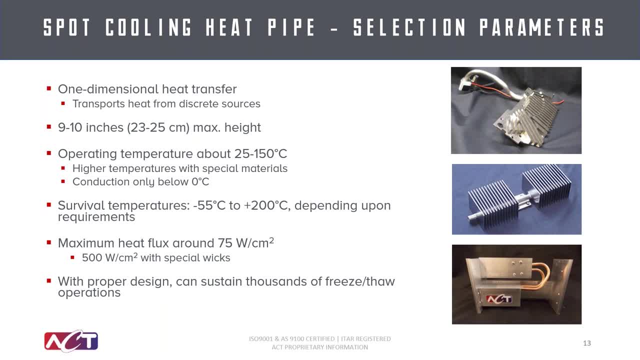 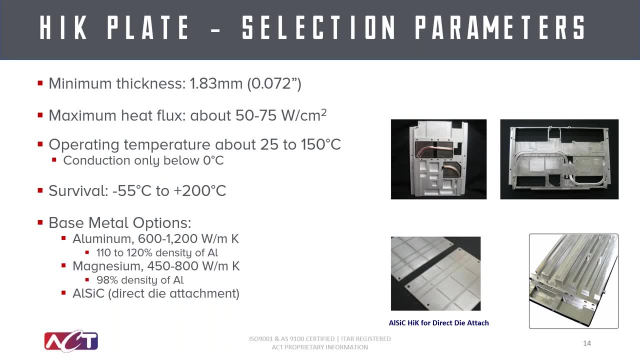 flexibility and and ability to retrofit heat pipes into designs is one of the reasons they're you so much. the next integration we'll talk about for heat pipe technology is high k plates or high thermal conductivity plates. these are one of the more commonly used situations in aircraft because 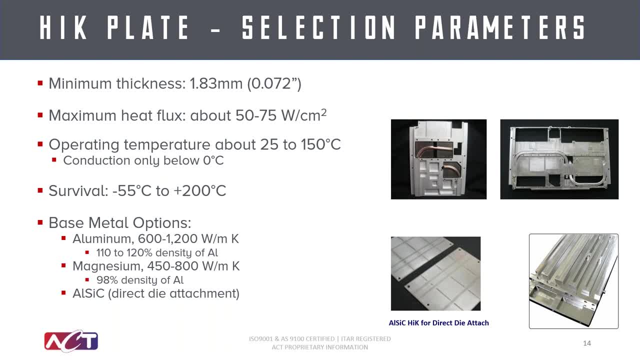 they. there's a lot of heat spreaders already designed and by implementing heat pipes you just increase the thermal conductivity of those heat spreaders. so again for aircraft applications. you want to keep the mass low, so a lot of these type of applications look to have a in a spreader as 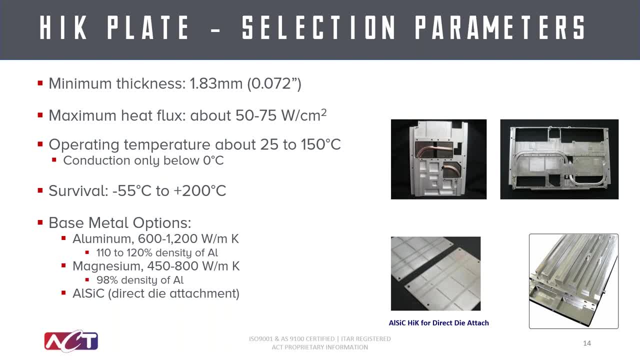 possible, and we've gone down to under two millimeters, 1.83 millimeters and in thickness, with embedded heat pipes. again same heat flux capability as the standalone heat pipes, same operating temperature range, same survival temperature range, but at the end of the day, what you get is is a heat spreader. 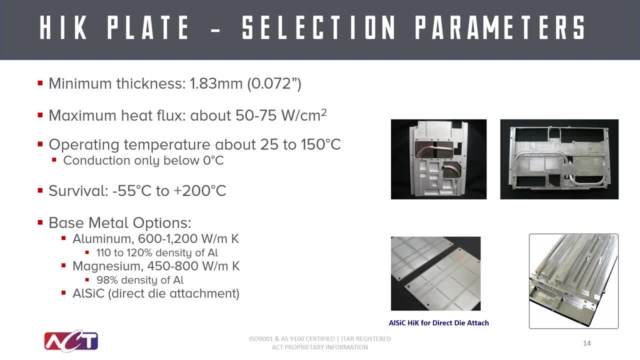 two-dimensional heat spreader with thermal conductivities much improved from the base metal. so we talked about early on the base metal, aluminum being about 167 watts per meter K in the. in these high k plates you can get that to 600 to 1200 watts per meter K and again aluminum's much. 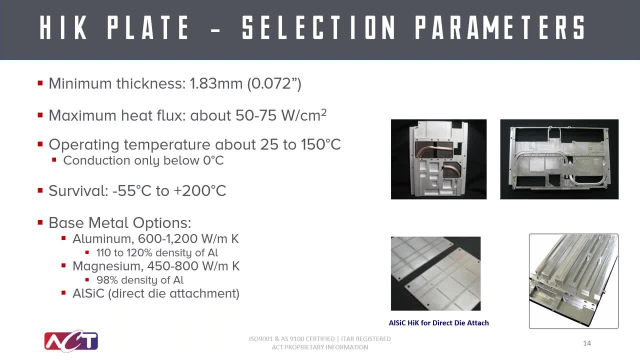 preferred. it's easy to machine, it's lightweight, it could be used as a structural component, so that is by far the most common, and you get a lot of advantages by integrating heat pipes into those others that we've used in the past for Aviation, magnesium for for the lightweight, so a slightly 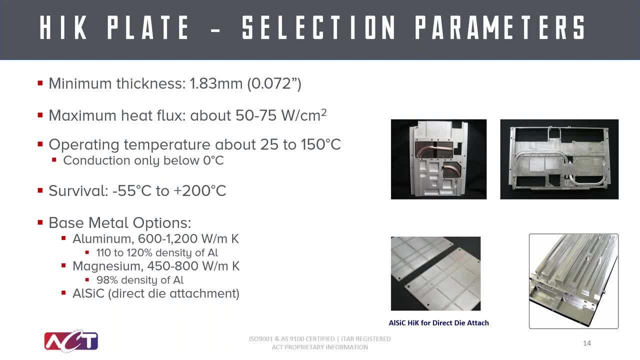 lower density than aluminum. um, let lower thermal properties, but uh, if weight is is more of a premium than thermal performance. magnesium is a good option and then ALSIC, so aluminum silicon carbide that can be used for low CTE or direct mount applications, and again, you can see a picture there in the lower left, but we can embed heat pipes directly. 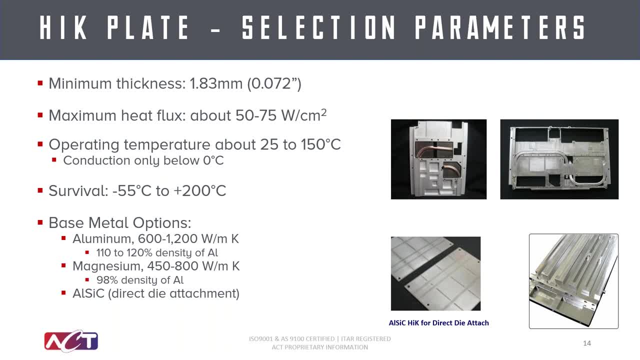 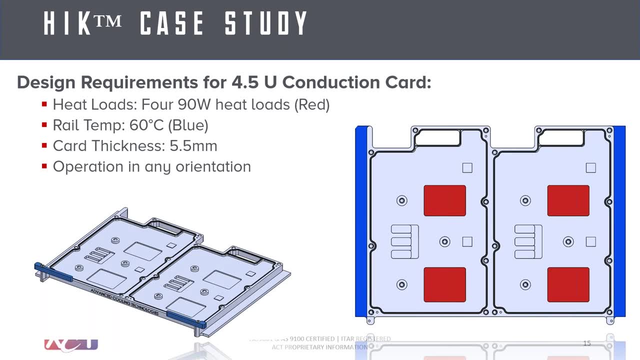 into the, the ALSIC, and have a kind of nice smooth spreader for for those type of applications. now I'll talk about one quick case study here and show you how these are implemented. so this is kind of a pretty standard. design too will get specced at ACT. so in this case you had a 4.5 U card. so 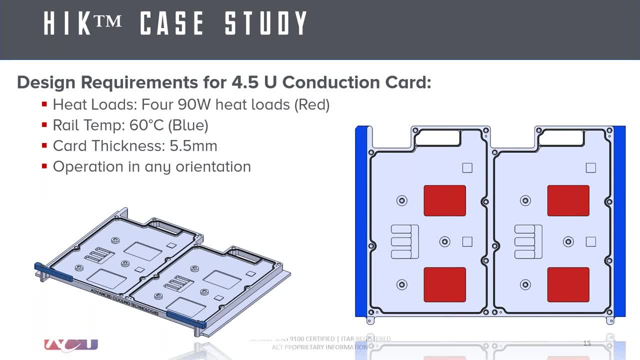 that's. that's basically the form factor of the card. um, you have four heat loads that are 90 watts. you can see them spread out there in the the red squares. in this case we had a rail temperature of 60 degrees C, so you assume there's some liquid cooling going on at the rails on or on the side. 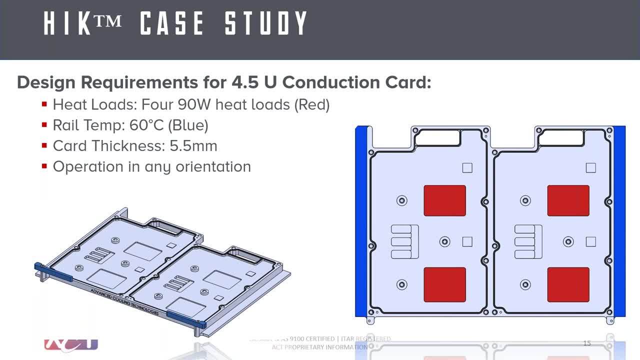 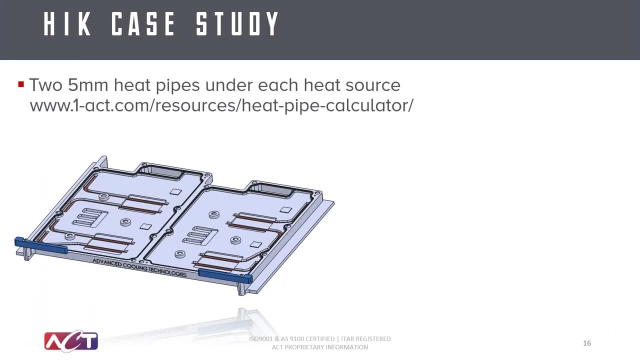 walls of the chassis, so we're designed to a 60 degree C rail temperature. you had about five and a half millimeters for room to embed heat pipes and this needs to operate in any orientation, which is a pretty typical design requirement. so we looked at running the the first. 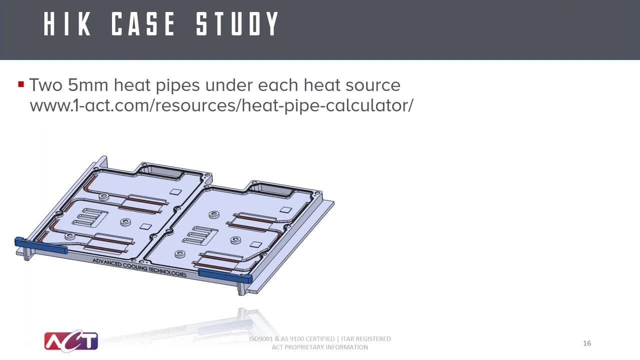 thing to do is size the heat pipes for the power capacity. so one of the tools we have- that we won't run through an example, but it's on our, our website if you want to go play around- is using our heat pipe calculator to size the heat pipes. so in this case, we found that putting two five millimeter. 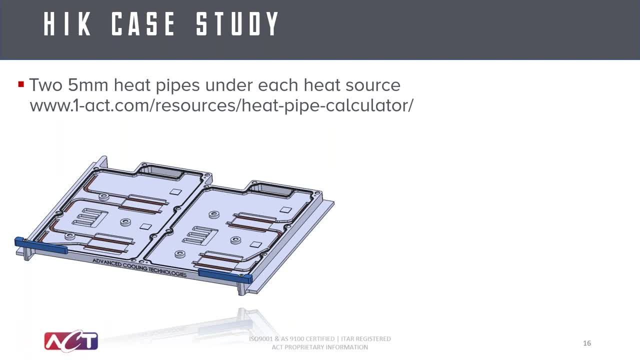 heat pipes under each source gave you enough capacity to move the heats and from there it was a matter of strategically placing the heat pipes to spread that heat along the rail as much as possible to lower the heat flux into the next higher level assembly. so there's a couple different. 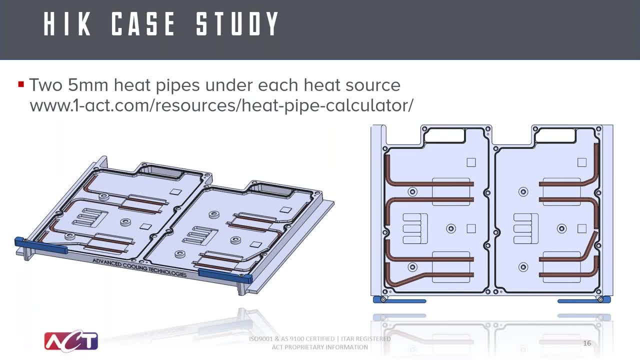 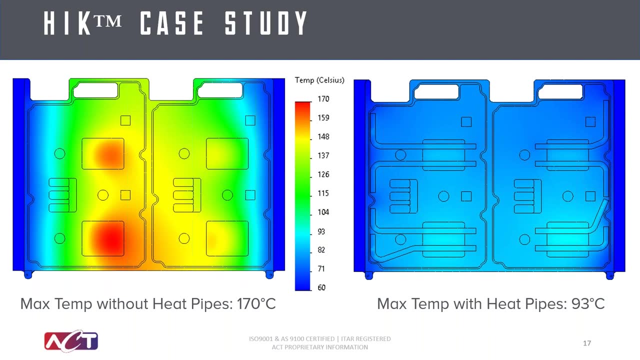 schematics you can see. um, yeah, the strategy here is just get the heat out to the edges as efficiently as possible and then route along the edge to get as much surface area as you can. and here's the before and after the picture. so before implementing heat pipes, they were running their their case temperatures. 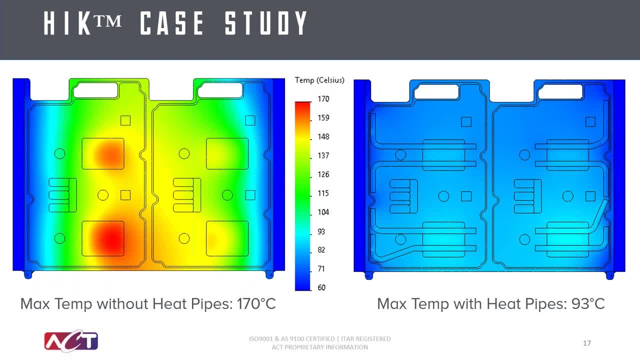 at about 170 degrees C. so if their criteria was to design to that 135, they were exceeding their max case temperature. by embedding heat pipes you're able to greatly drop that down. they ended up with a 93 degree C case temperature here, so meeting the criteria with pretty significant. 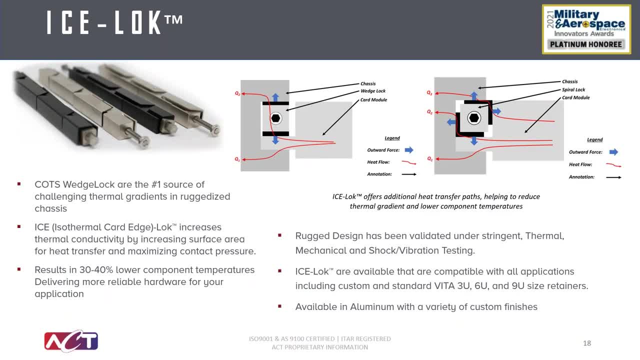 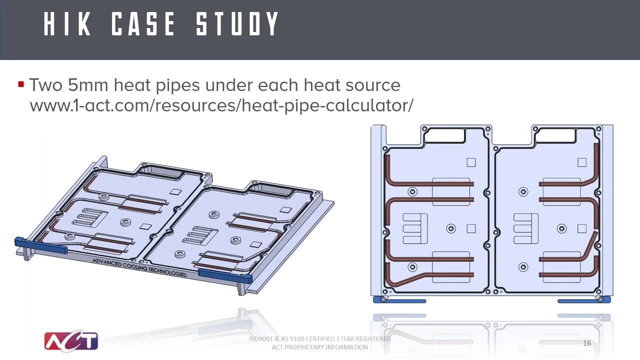 margin there after implementing heat pipes. um, the next thing we'll talk about here is again other enhancement to conduction systems. I'll go back to to this example real quick here. so in many of these avionics applications you have cards that slide into chassis and at the rail right. 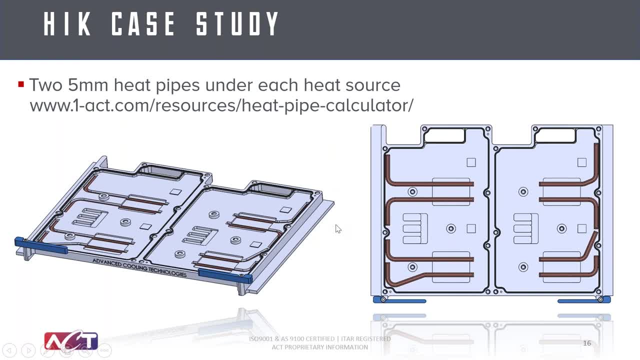 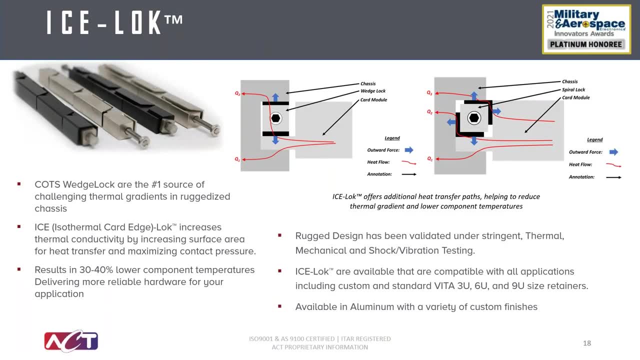 here, if you can see my mouse- you're implementing a wedge lock and that gives it a mechanical joint to the chassis and also gives it a thermal path to transfer heat to the chassis. the challenge with traditional wedge locks is there's a pretty torture of a cooling process. so if you don't have a traditional port, ready to move the get to the house, even if you have camera or a device that can be installed, and that's not a challenge because that's two or three different ways of doing it, but that's what's the challenge. we look at a couple of options and one of the challenges is if you're 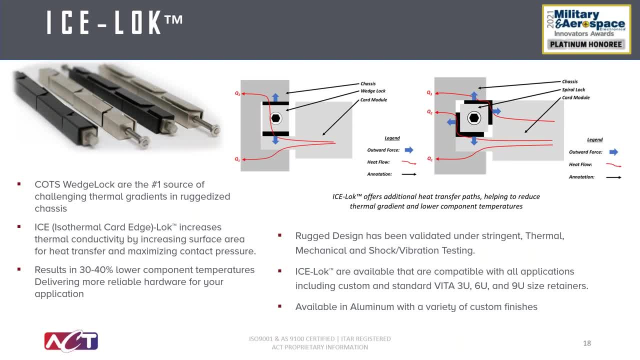 a fan of preferential refrigeration or you're a fan of heat, from heat, and you could be a fan of air and knowing that this was your pretty important, especially when you can always use a driving system, thermal path. so with the metal, the metal interfaces of wedges pushing together, it's not a great thermal. 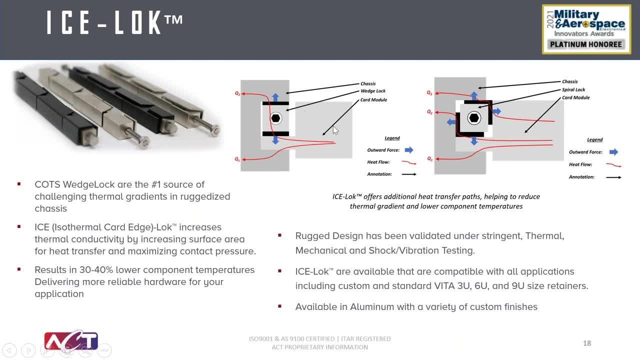 path to go through the wedge lock. so in in the case of a traditional wedge lock, which you can see here to the left, about 70 percent of your heat is dumped straight from the board to the chassis, because that's the lower thermal resistance path, through the wedge lock itself. you have 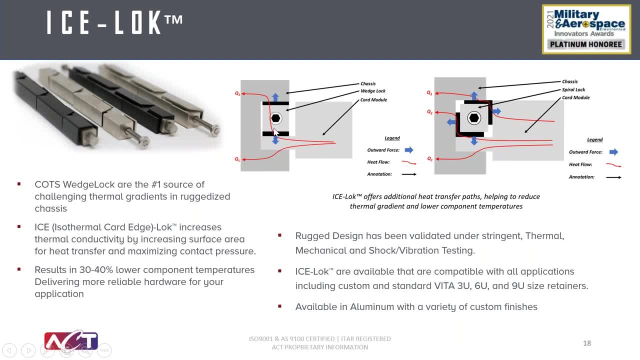 metal metal interface, both at the card edge and chassis, and then you have a couple different metal to metal interfaces to the wedges themselves. so overall it's a. it's a small thermal path that becomes a bottleneck in the system. so what act designed and patented was? 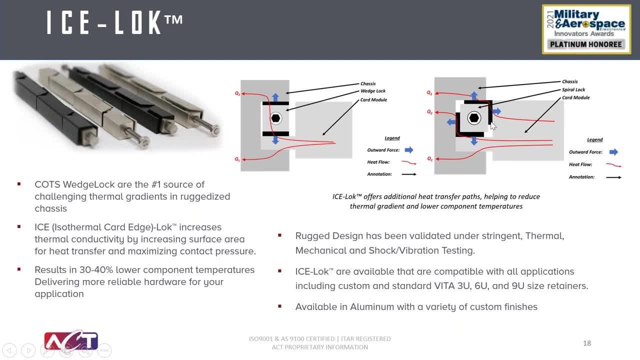 an ice lock which expands in all directions, so it adds additional surface area contact points on the card frame and an additional contact point on the chassis and creates kind of a third unique thermal path directly through a single wedge to the chassis- uh, through a single wedge to the 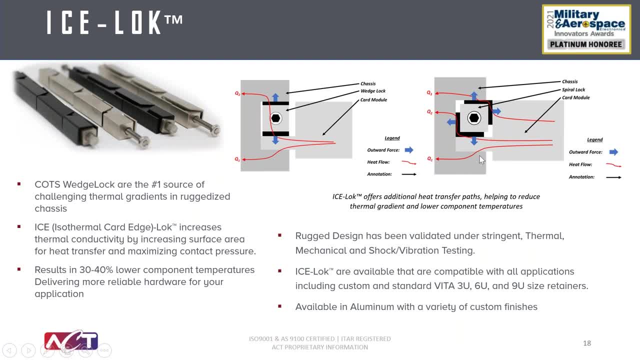 top of the chassis and then the bottom of the chassis, and then the bottom of the chassis and the top of the chassis, and then the same path through the board frame to the chassis itself. so adding additional surface area and another conduction path was able to drive those that. 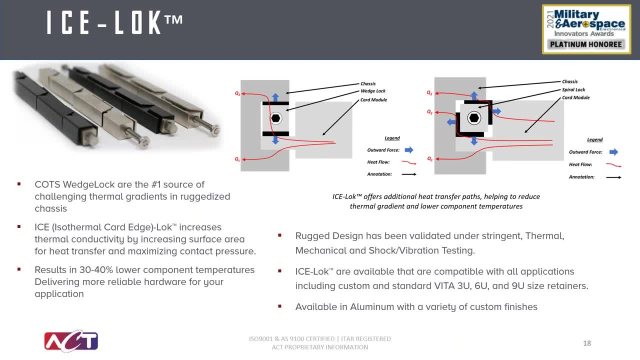 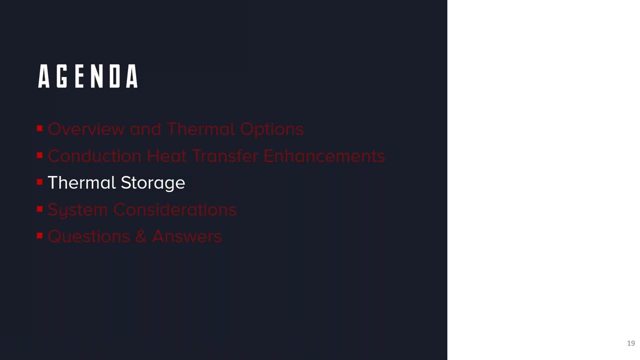 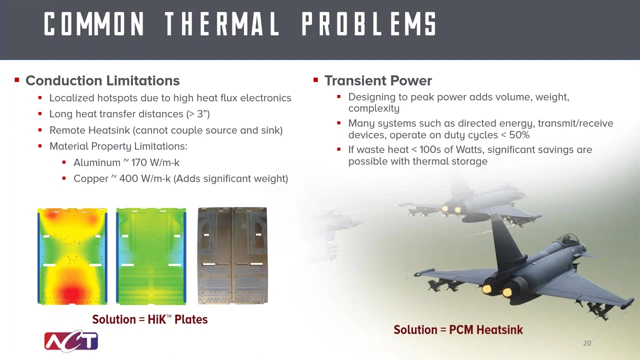 thermal resistance at this joint, which became a bottleneck, down by about 30 percent, so a significant reduction in delta t across this joint, which again could lead to higher performance, as these are implemented into systems and every degree becomes pretty precious. the next thing we'll talk about is thermal storage. so we talked about conduction limitations. now we'll talk 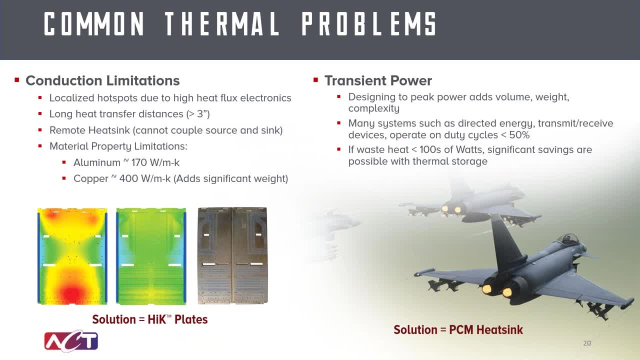 about transient power. so in many cases the electronics or systems that you're operating for an aircraft will not be on all the time, and if they do run on significant duty cycles, one of the things you can do as a design engineer is absorb that during the on period and then dissipate. 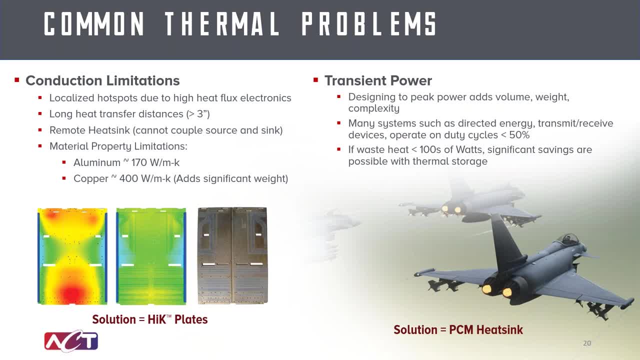 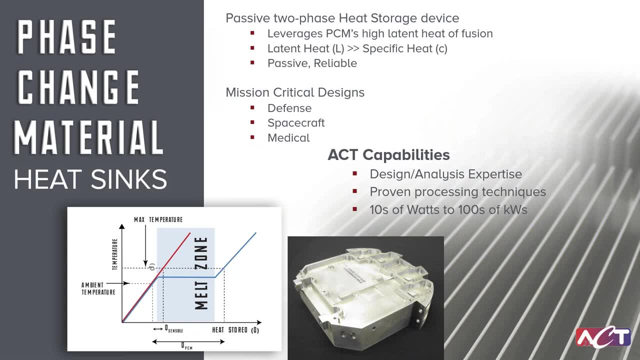 it during the off period and that allows you to greatly reduce the overall size of your ultimate heatsink, because you're designing to average power instead of peak power and the the way you do that is using phase change material or a thermal storage device: pcm thermal storage device and the 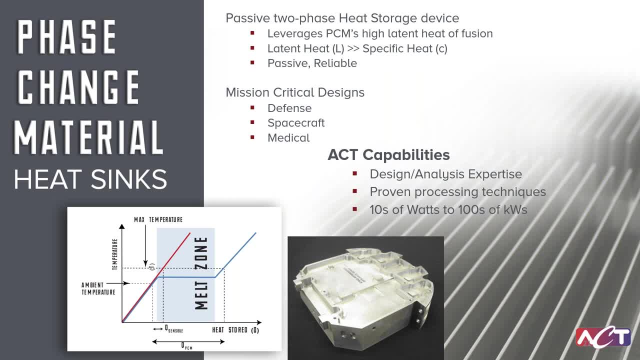 the way these work is: during that melt phase, that's, solid to liquid transition, you use the latent heat of the pcm and that latent heat is an order of magnitude plus of the specific heat of a metal or the material itself. the other big benefit is these are passive solutions. again, no moving parts. 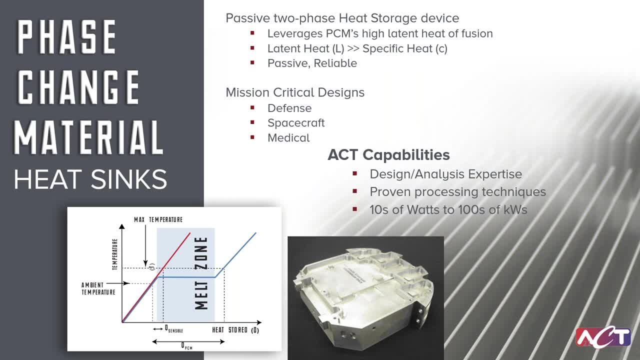 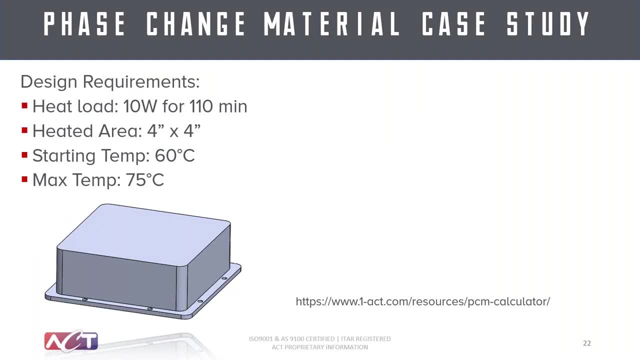 highly reliable and fairly simplistic systems, and by taking advantage of that lane heat range you can again greatly reduce the downstream size of your ultimate heatsink. so we'll talk about one example here. this is an example where you have 10 watts for 110 minutes. this was a case where you had a single type mission, where you basically need to serve a 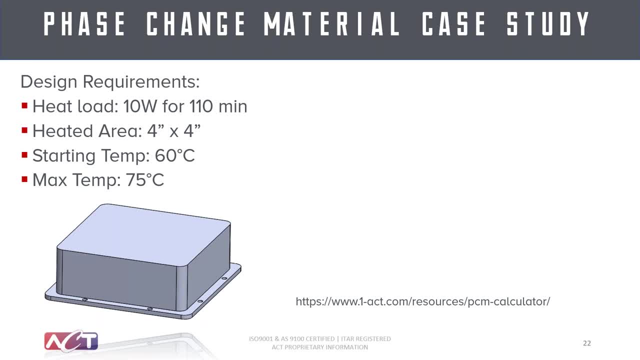 110 minute mission, but again, designing a complex thermal solution for for that, as opposed to just dumping the heat into a pcm, makes it a lot more challenging. in this case there's a four inch by four inch area, starting temperature of six degrees c, and they need to hold the, the electronics, to not 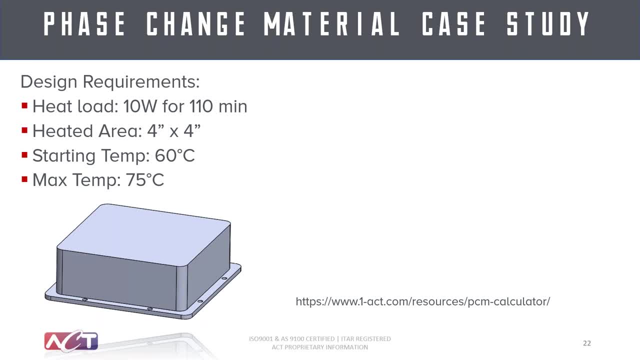 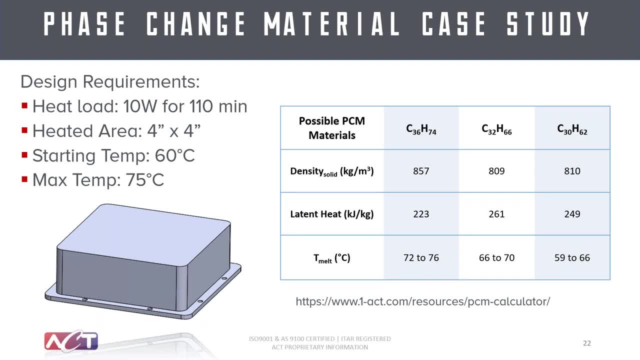 the specific heat before and after. you need to make sure you don't exceed that 75 degrees c. so here's a couple different options that that we came across. basically, looking within that, that melt temperature range, and you can see the latent heat associated with those different materials. so this: 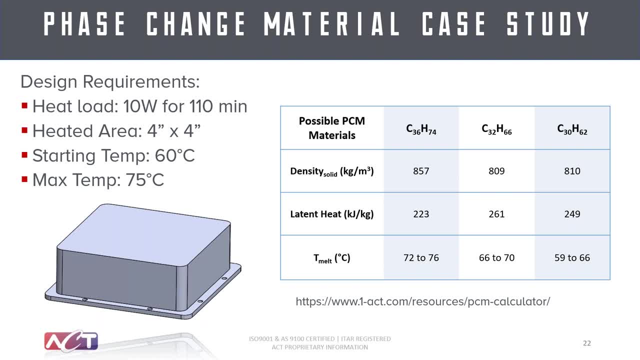 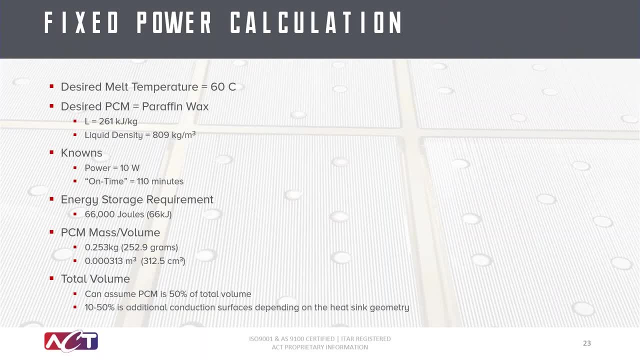 is kind of with the trade-offs between density, latent heat. you want your latent heat as high as possible, density as low as possible, and then the melt temperature needs to be within your- your requirements- range. so we're going to talk a little bit about the data. so we have a similar: the pcm and the pcm. 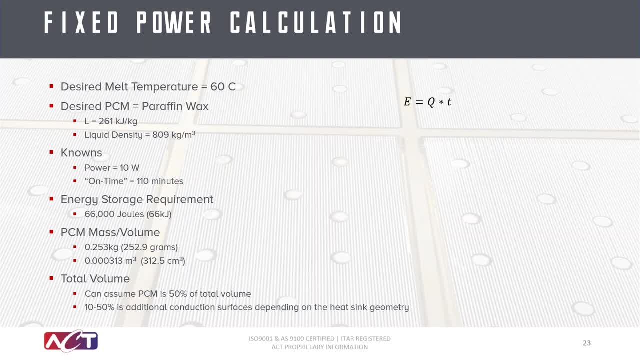 matters if you're looking to cold water storage in a room with a similar size in your system. so this is going to be a really interesting plot of how you can measure and you can see that just by touching on a piece of the picture on the fly. like this is the on time of the on-time. 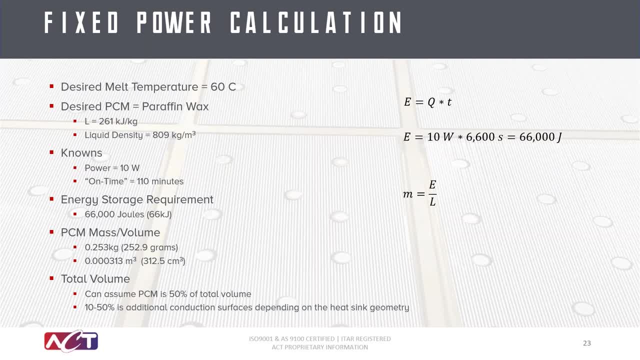 temperature of your site. so we're going to talk a little bit about the on-time temperature, the current temperature time, on-time temperature of your site. so we're going to do a little bit of modeling over here. so this is just showing. just look at what's going on in our pcm plate. so the temperature is the amount of pcm we're using in our pcm, as well as the density, and that's the same thing for a solar unit. we have a lot of energy for the solar unit and then, so we're going to check out what changes there are here. 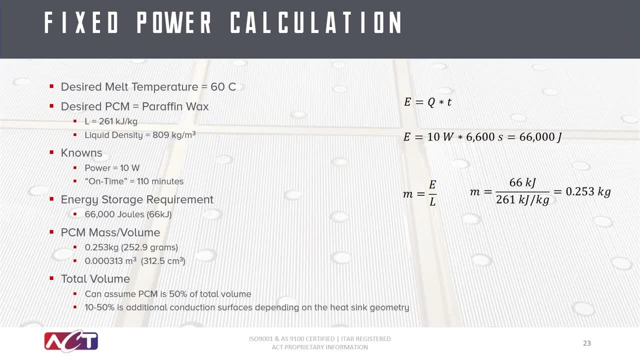 of your PCM. so the one we selected here had a 261 kilojoule per kilogram latent heat, and that results in about a quarter kilogram worth of PCM, and then you can kind of determine the the volume required, and then, based on your footprint, you can size out the height of the PCM. 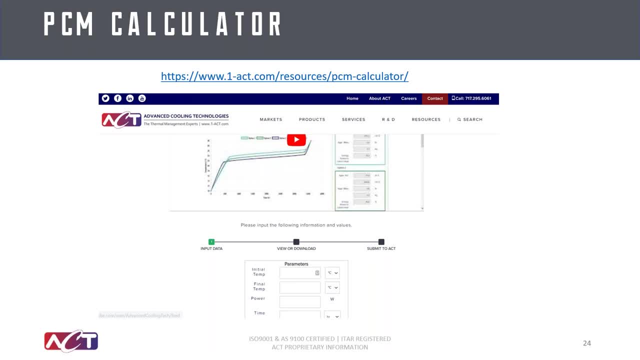 now, that's kind of the quick calculation. to do that, another resource we have online is our PCM calculator. so the big advantage here is we have a large library of phase change materials. so it'll select the appropriate based on your temperature ranges, based on your power levels. 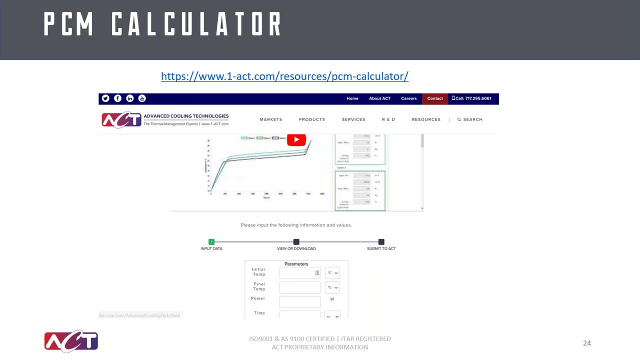 and it'll output a couple different options for curves which then you can use to design your system, and this will also kind of account for the envelope material. so the mass output here will account for not only the PCM but also the enclosure itself, which uses some general 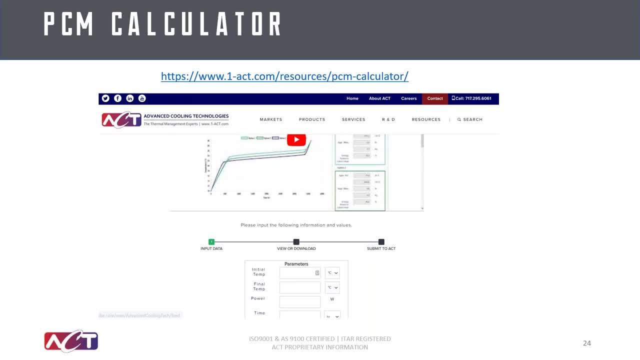 guidelines and can most of the time be used for the PCM, and so that's kind of. the big advantage here of the PCM is that you don't have to have a lot of thermal conductivity to be able to use the PCM. so you don't have to have a lot of thermal conductivity to be able to use the PCM. 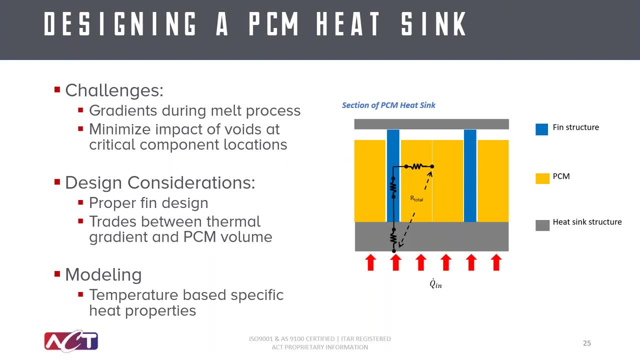 and then taking it one step further. this is where kind of the uniqueness of the design and modeling comes in. so the big benefit of PCM is the high link heat capability, but the challenge is the very low thermal conductivity. so from a design standpoint you need to have conduction pads that are robust to melt the entire volume of PCM. 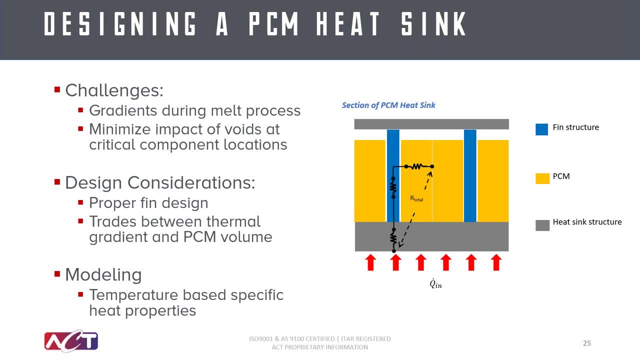 as opposed to localized melting where you might run thermal runaway trying to conduct through the the patient material with that low thermal conductivity. so a lot of times this is done through metallic structures, spin structures internally. it can also be done with significant enhancements, such as heat pipes which are kind of a superconductor. but overall you need to model. 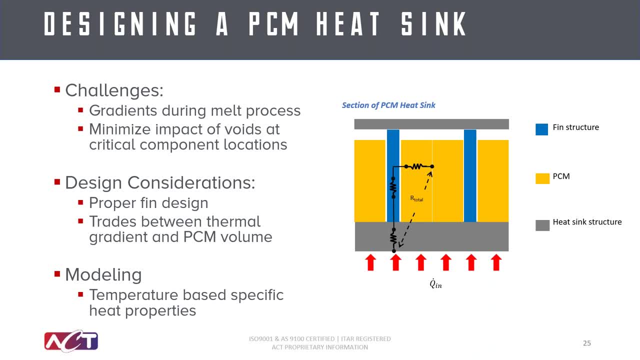 these properly to make sure you're melting your entire PCM, and one of the techniques to modeling is using a temperature based specific heat problem, which is the heat that's going to be used to melt the entire PCM, and one of the techniques to modeling is using a temperature based specific heat problem, which is the high link heat capability. 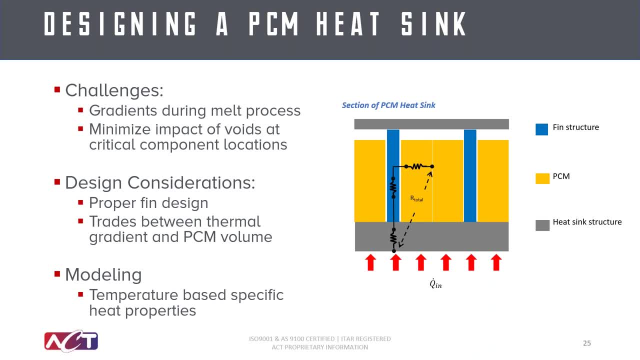 and one of the techniques to modeling is using a temperature based specific heat property. so, similar to modeling heat pipes where you adjust the bulk thermal conductivity, um, in this case you're you're modeling where you're just changing the specific heat of the material based on temperature range. so when it hits the melt temperature range you spike up. 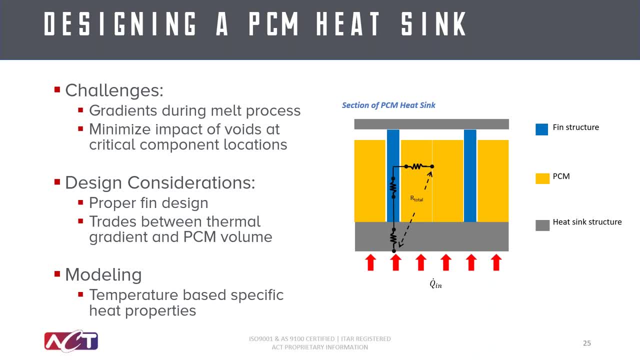 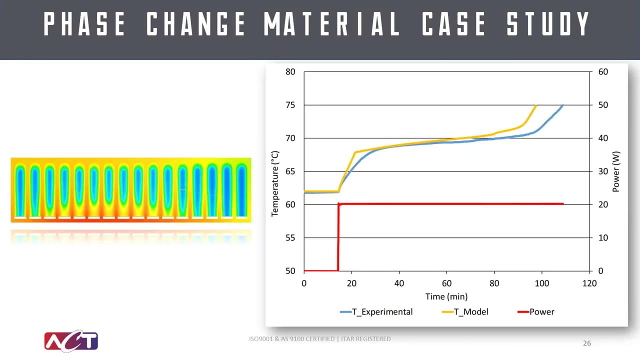 the specific heat of the material and then when you hit the full liquid range it spikes back down and that that gives you kind of a general way to model these. but the big, big challenge is the conduction pads, getting the heat into the PCM itself. and here's just kind of an example of a model versus experimental results so you can see your. 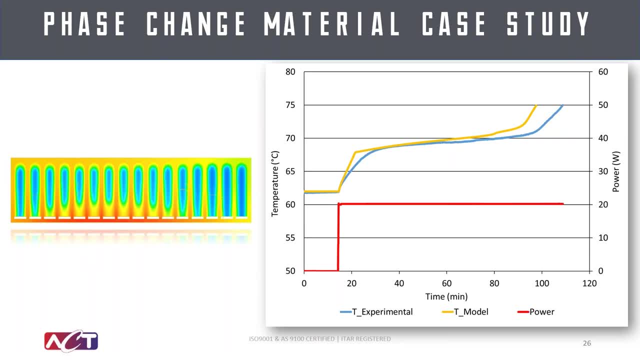 modeling will typically have kind of some rough corners associated with those spikes in your specific heat and the experimental will have more of a smooth, as you have the secondary conduction paths. but overall the modeling can can match your results fairly, fairly accurately. so again, if you're 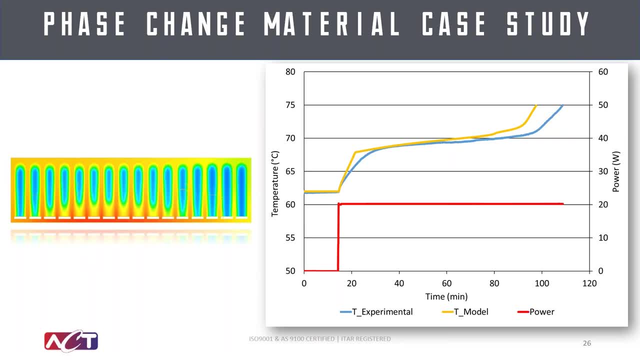 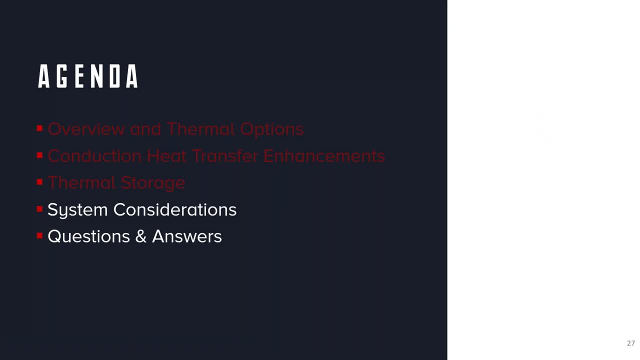 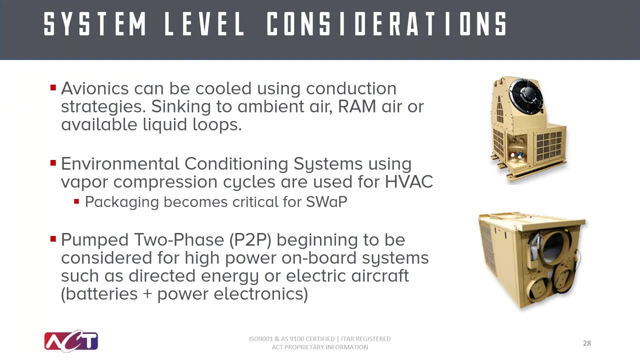 looking to model these systems that need some support. this is something where ACT has a lot of benefit. next we'll kind of just wrap up with some system level considerations and then go to some Q&A. so just one slide here, not not diving into any large details, but if you do have system level, 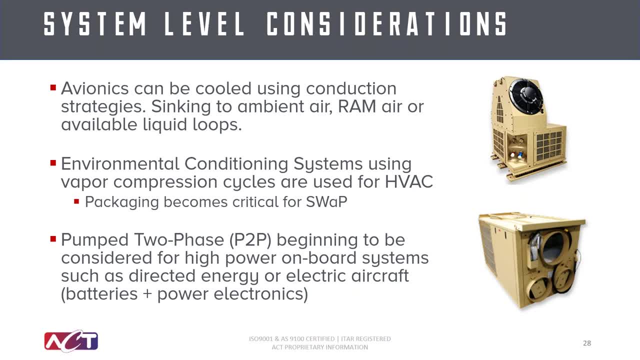 considerations. the focus of this webinar was on the avionics side, but if you do want to talk about the overall system, whether it's liquid pool, whether you're doing ram air, please reach out. we have a lot of experience in those systems as well, but again, today was more focused on the the 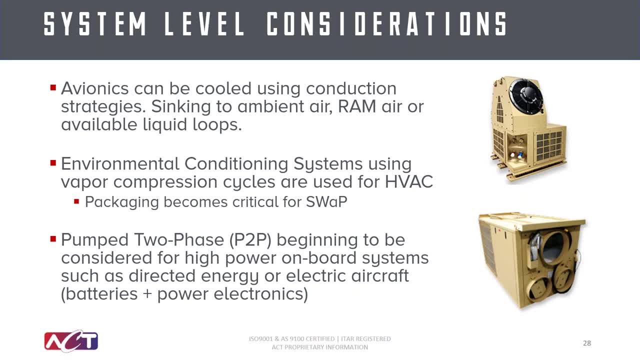 system as well: the avionics boxes themselves and getting heat out from your component level electronics, but in general, system level considerations- is understanding your sink, whether it's your ambient air moving into the skin of the aircraft, whether you're leveraging or ducting ram air into the system. 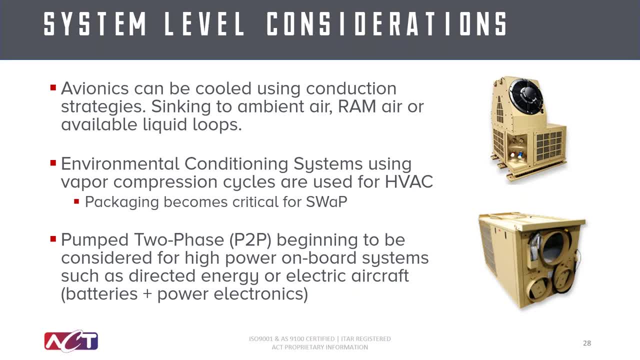 or if you're coupling into the liquid loops that are available for some of the primary coolant systems or or fuel systems. another area- that's is a big design criteria for these type of aircrafts, especially some of the newer electric vehicle aircrafts or eb tolls- is the environmental. 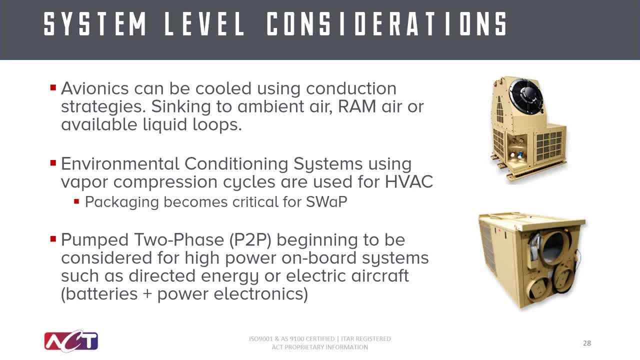 conditioning system. so this is used for basically your hvac system, using vapor compression cycles to kind of optimize the um the environment within the aircraft itself and coupling your, your electronics cooling to the. the ecp s is also um a strategy used a lot but you don't want to dump too much heat because 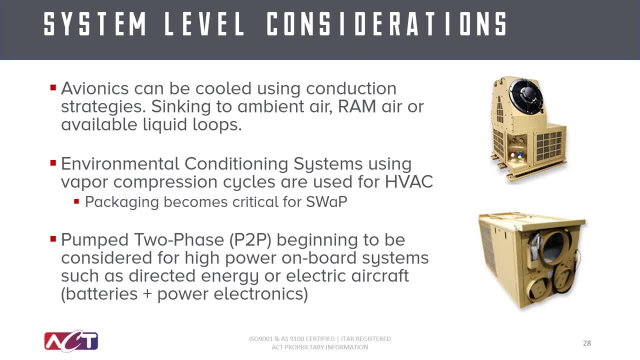 um, you want to get as much heat off board as possible, not not oversizing your ecs, because vapor compression is a little more robust of a system, could add a little more mass. so that's where packaging becomes critical for size, weight and power considerations. and then just want to touch on again. if you have more questions, we have a lot of resources on. 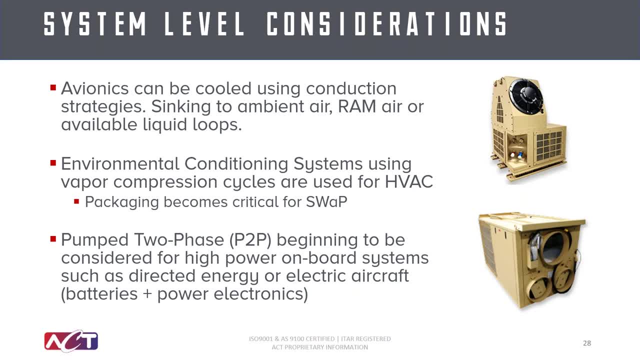 pump two-phase technology, but this is beginning to be considered in aircraft applications for higher performance aircrafts, so we're going to talk a little bit more about that in just a moment. so if you're looking at a round trip or a test flight where you have a lot of time to take, 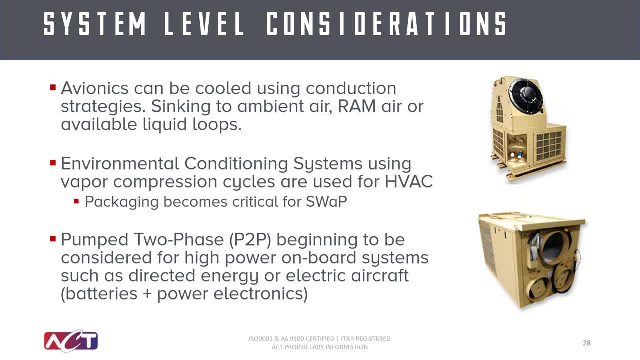 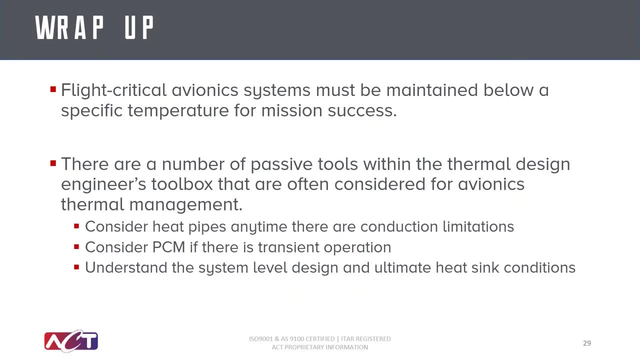 your flight at a high speed or you have a lot of power on board systems, especially in military aircraft that are looking at like direct energy or some of those commercial all-electric or hybrid electric aircrafts where they have a lot of batteries and power electronics systems in there. 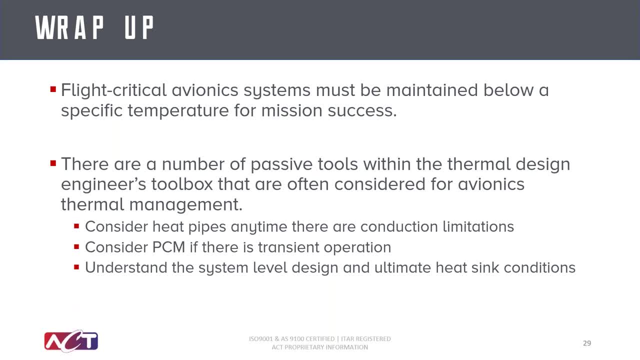 so with that we'll kind of wrap up and hopefully we got some good questions here and we can take those. um, but just to wrap up, flight critical avionics must be be maintained below your understanding. your sink conditions is pretty key and hopefully you came away with a number of. 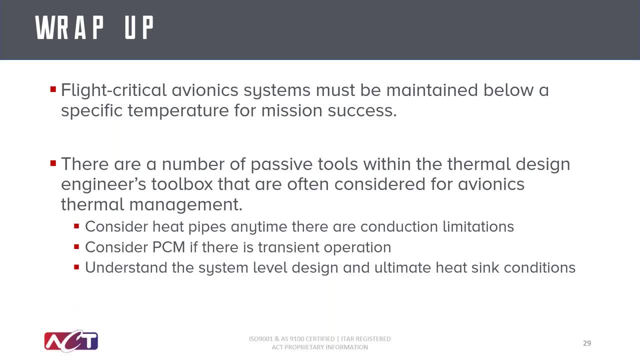 passive tools within the engineers toolbox for consideration here. the big things that we talked about, our heat pipes- consider those. anytime conduction limitations are a big factor in your system. and then phase change material. any times there's transient operation on off cycles or short-term electronics that are just on for a short period of time, PCM can absorb the thermal.